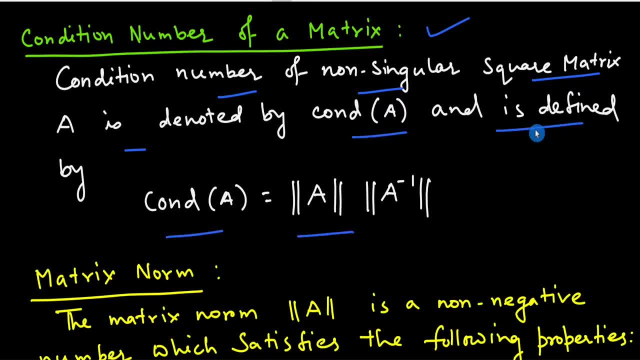 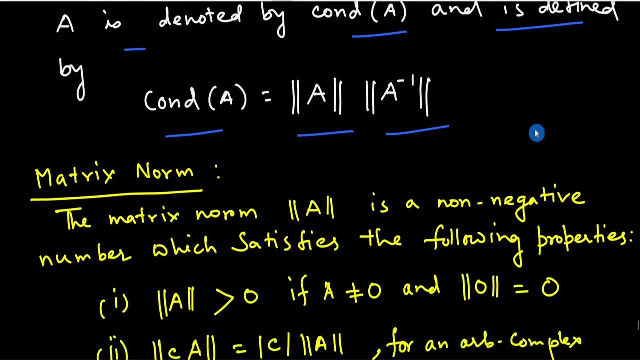 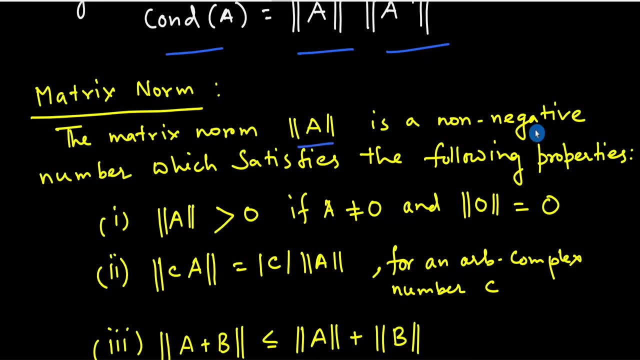 is defined by condition of A equal to norm of A. Now we will define first the matrix norm for this condition number. So matrix norm, the matrix norm, mod of norm of A, is a non-negative number which satisfies the following properties: Properties number one: norm of A is always greater than zero if A not equal to zero. and. 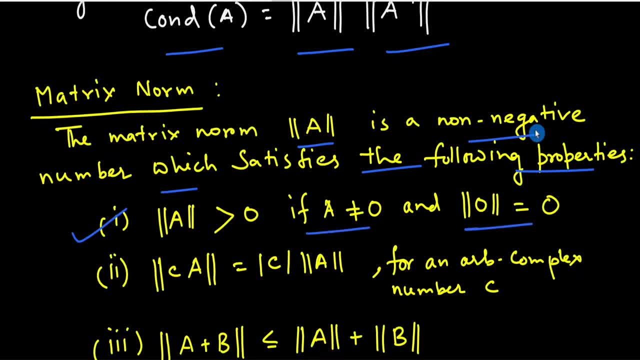 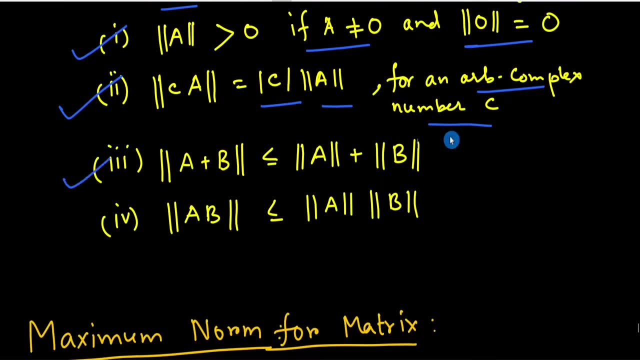 norm of A equal to zero, if, and only if, A equal to zero. Condition number two: norm of C: A equal to mod of C into norm of A for an arbitrary complex number, C. Condition number three: norm of A plus B less equal to norm A plus norm of B. And condition number four. 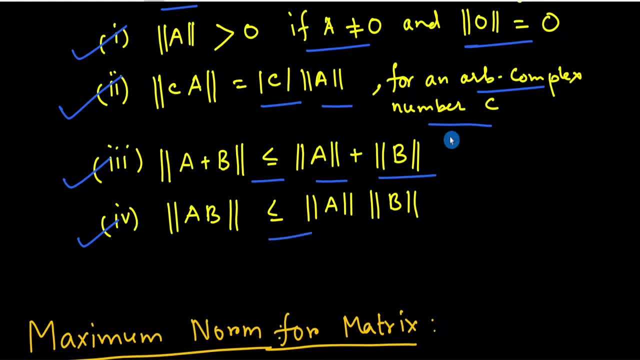 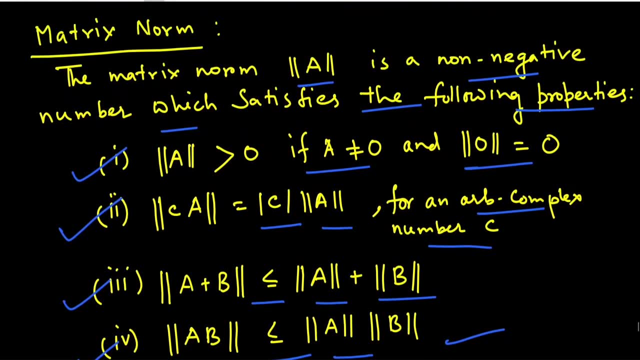 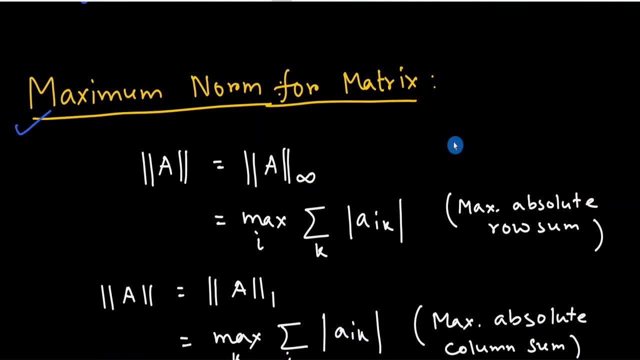 that is the last condition, is norm of A, B less equal to norm of A into norm of B. So this four condition, whether this four condition satisfies, then we define the matrix norm, So that the matrix norm, which is called maximum norm for the matrix, Now this norm of a matrix, 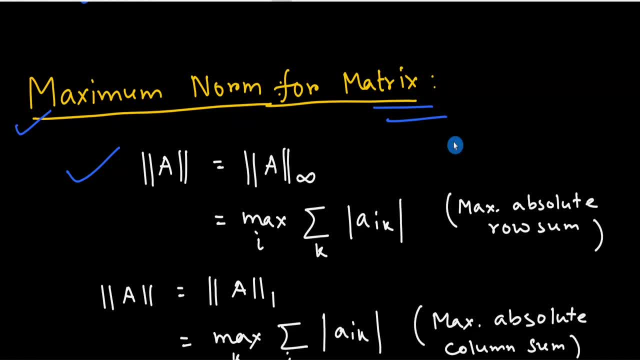 equal to. we will say that it is called infinity norm, and norm of infinity equal to max of I. summation over K, I A, I K. That is the maximum absolute row sum. This is the maximum absolute row sum And similarly norm one that is norm. 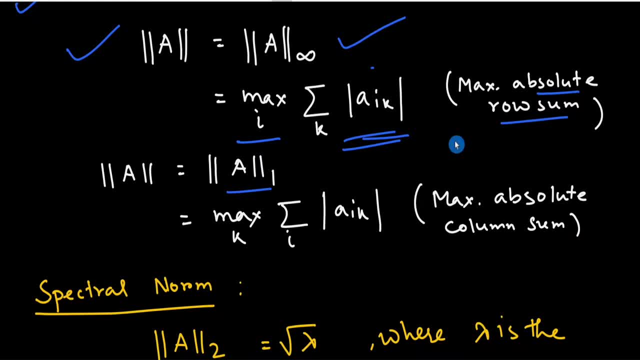 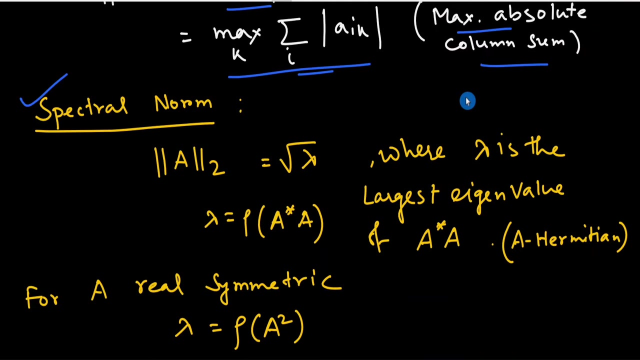 Of a matrix equal to maximum of K into summation of A I K mod of A I K. That is maximum absolute column sum. Therefore, by means of infinity norm we define this And in case of norm one, then we defined column sum. Now we define the spectral norm as norm of A2, equal to root. 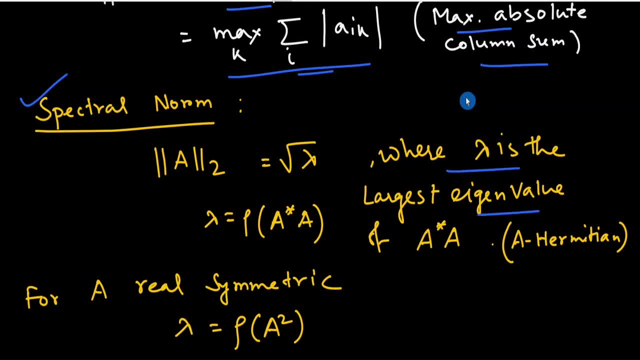 under of lambda, where lambda is the largest eigenvalue of A2.. We now define the spectral norm as norm of A star eight, where this A is the complex matrix Now lambda equal to. we define row of A star eight. Now for a real symmetric. 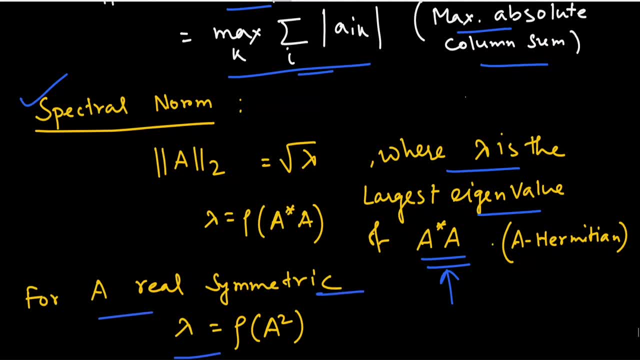 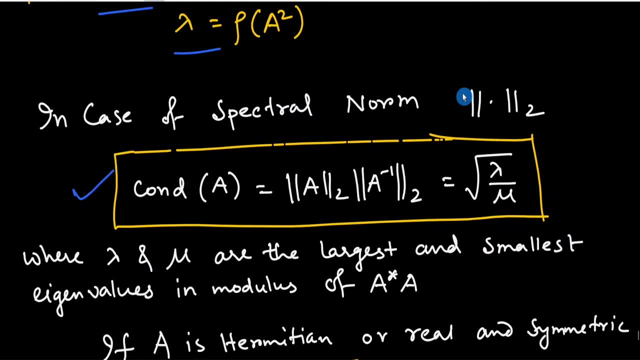 matrix lambda equal to row of A square. Now, in case of spectral norm, norm two, condition number is defined by condition. number of A is equal to norm of A2 and norm of A inverse two. This is equal to root under of lambda by mu, where lambda and mu are the largest. 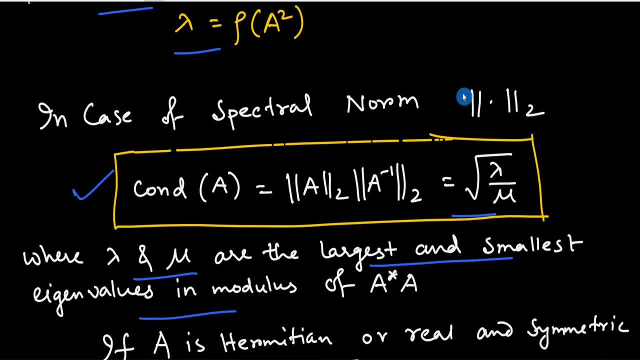 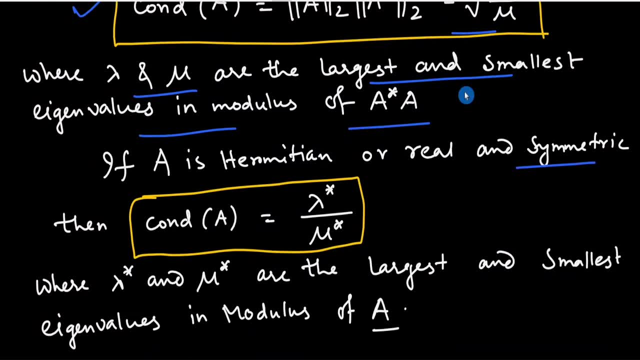 eigenvalues, largest and smallest eigenvalues in modulus of a star, a. if a is a hermitian or real and skew symmetry as real and symmetry matrix, then condition number of a is defined by lambda star, by mu star, while lambda star and mu star are the largest and smallest eigenvalue in. 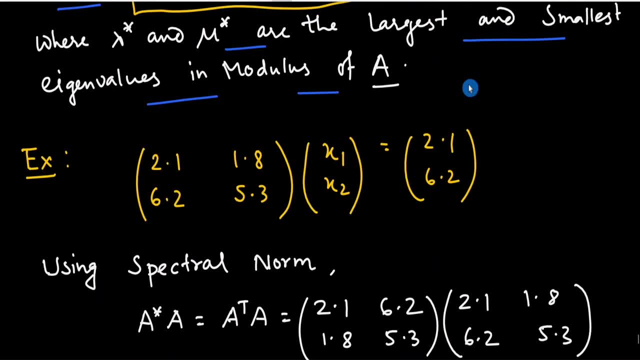 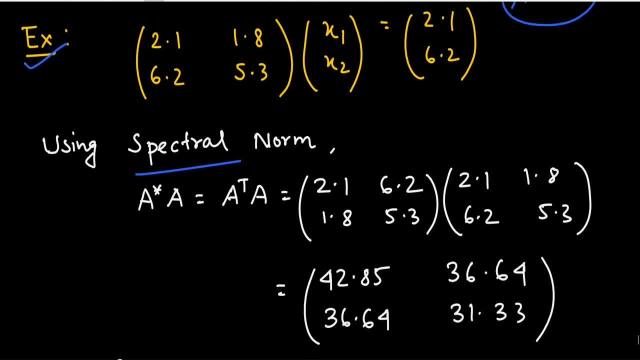 modulus of a. now let us take an example. this is a system: a, x equal to b. we have to find the norm of a with respect to spectral norm. now we first find the a, star a here, since a is real and symmetry real matrix. so we find a, transpose a, so this is equal to. we have 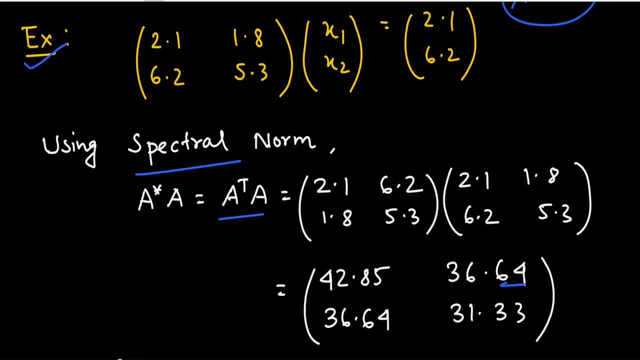 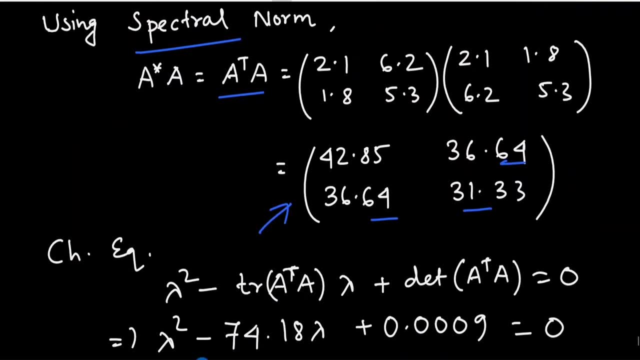 42.85, 36.64, 36.64 and 31.33. we note that this matrix is a real and symmetric matrix. now we find the eigenvalue of this matrix. so to find the eigenvalue of this matrix, we have the characteristic equation equal to lambda, square minus trace of a. transpose a into lambda. 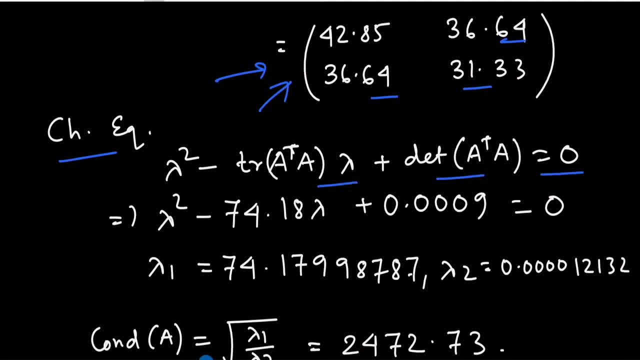 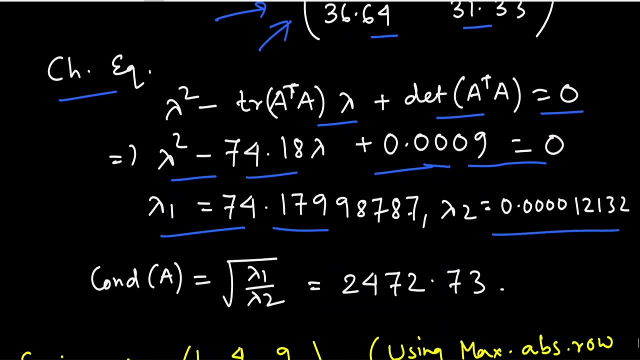 plus date of a transpose a equal to 0. this implies lambda square minus 74.18. lambda plus 0.0009. 0.0009 is equal to 0 and this gives lambda equal to this 74 point something, and lambda 2 equal to this now by the spectral norm, we have the condition number, which is: 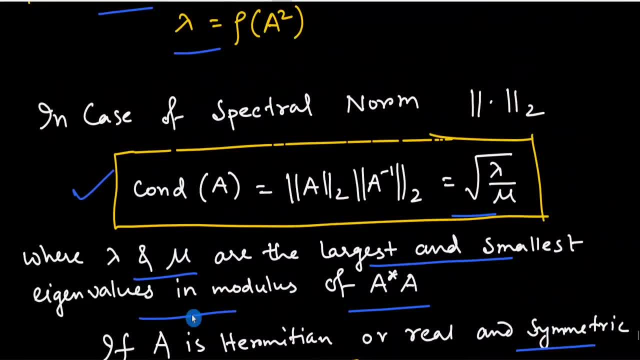 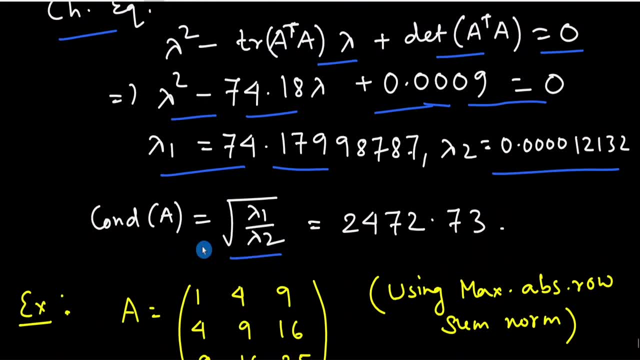 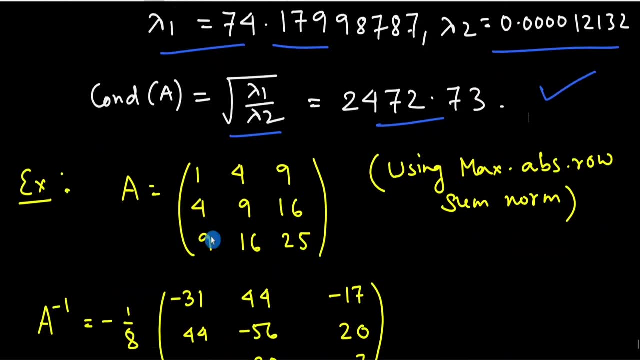 equal to root under lambda 1 by lambda 2. this formula: by this formula we calculate the condition number of this matrix, equal root under of lambda 1 by lambda 2, and this gives 2472.73. now example number 2: given a matrix, we have to find the condition number using the maximum. 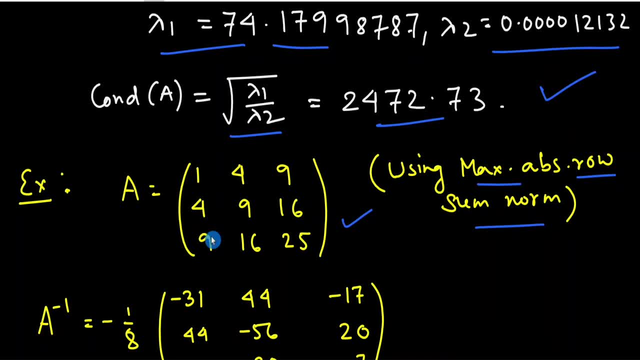 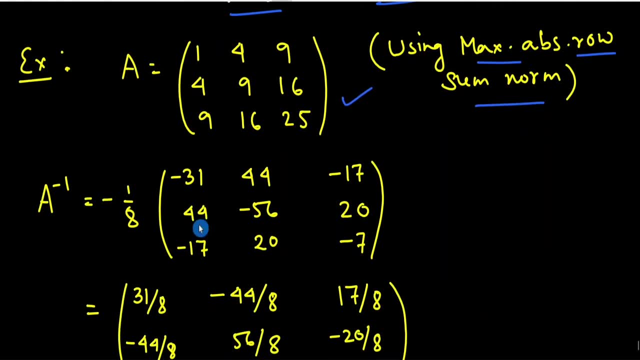 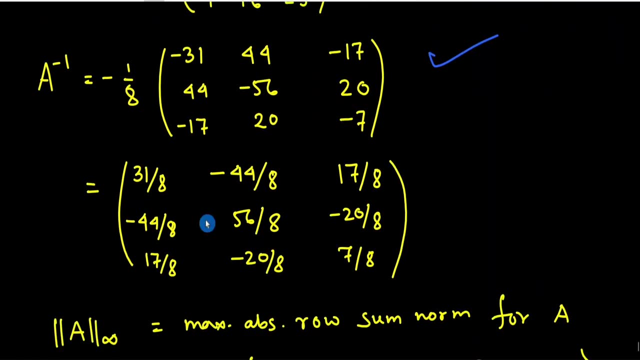 absolute row sum norm. that is using infinity norm. so a equal to 149, 49, 16, 9, 16, 25, and a inverse equal to this is simply calculation minus 1 by 8 into this matrix. now we can write this as a inverse equal to this matrix, that is 1 by 8 minus 44 by 8, and so on the matrix. 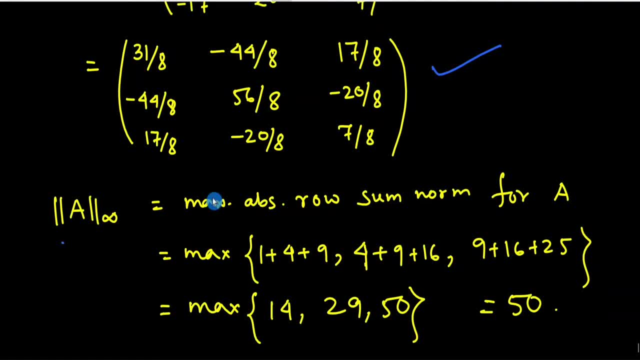 9 elements is here. so we now calculate the infinity norm of a, which is equal to maximum absolute row sum norm for a, and this is equal to maximum of first row sum, second row sum and third row sum. so these are the row sum which gives maximum of 14, 29 and 50, and 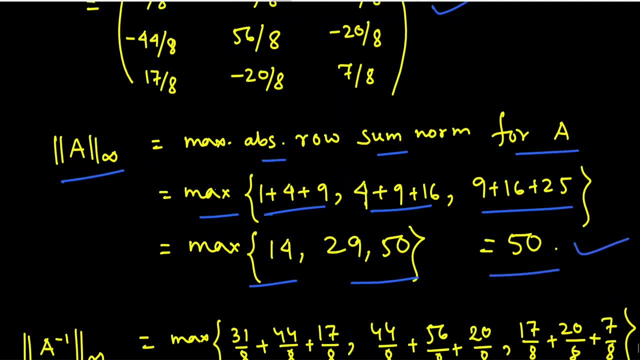 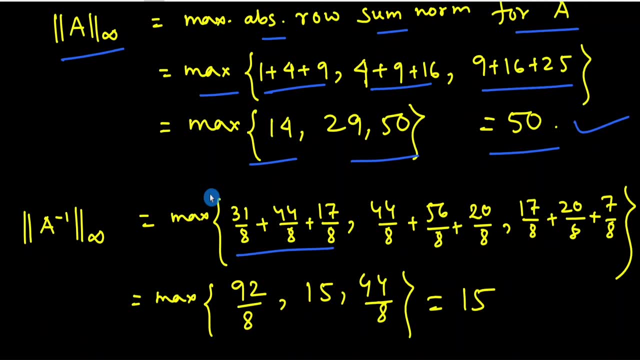 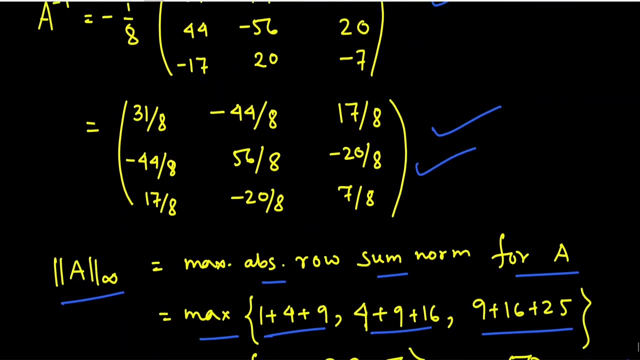 maximum of this is equal to 50. now we find the infinity norm of a inverse which is equal to maximum of first row, the absolute value of first row, elements of first row, the absolute value of elements of second row and the sum of the absolute values of the elements of third row. from this matrix, the absolute. 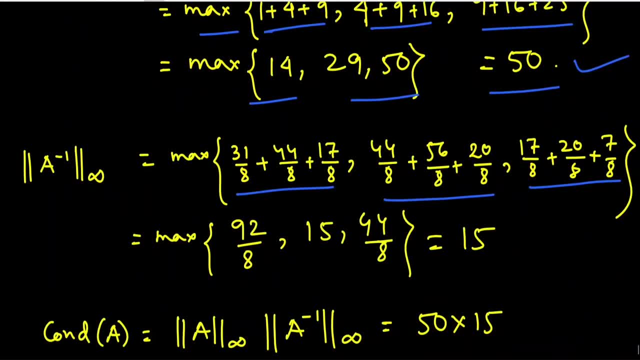 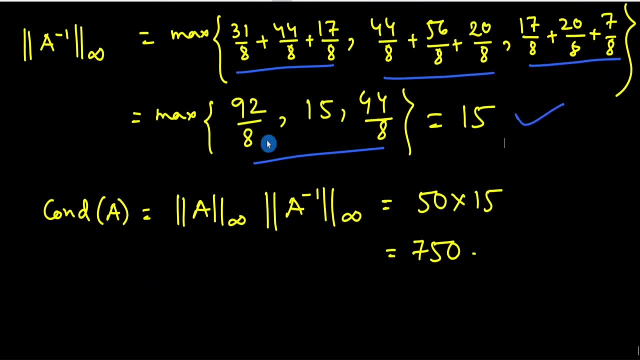 value of these elements and take their sum. so this is equal to maximum of these three and which gives the maximum is equal to 15. therefore, condition number of a is equal to norm of a infinity into norm of a inverse infinity. norm which gives 50 into 15, which gives 750, is the correct answer for this. 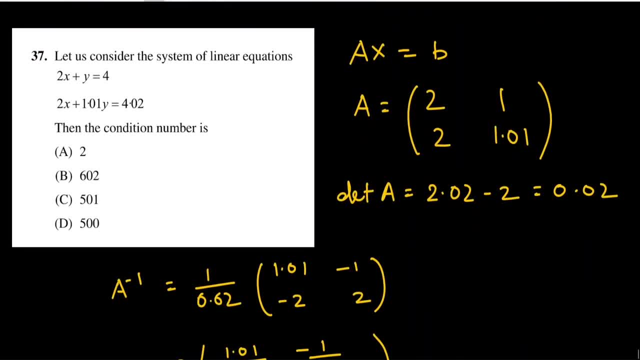 you matrix condition number. now we have another question, question number a question. this question is from WB set. I take this question from WB set question paper 2018. the question says that let us consider the system of linear equation, 2x plus y equal to 4 and 2x plus 1.01 y equal to 4.02. then the 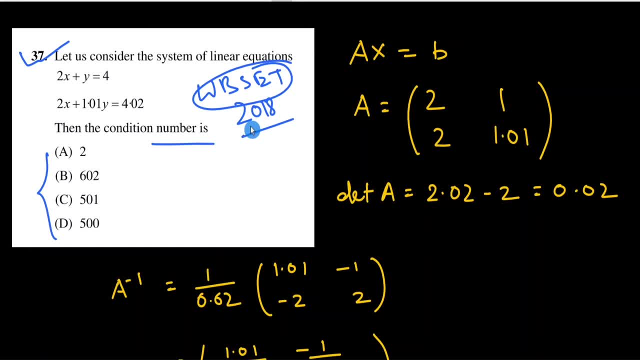 condition number is 4 option is pre given here now. the matrix a equals matrix a equals 4 option is pre given here now. the matrix a equals 4 option is pre given here now. the matrix a equals 2, a coefficient matrix is 2: 1, 2, 1.01. now we first calculate the determinant of. 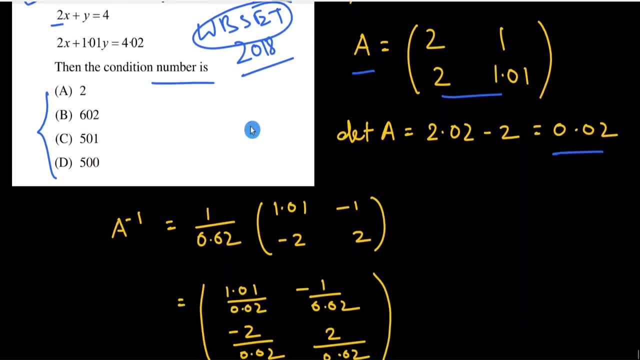 2. a coefficient matrix is 2, 1, 2, 1.01. now we first calculate the determinant of this matrix, which gives 0.02. now we find the a inverse, since we have to. this matrix, which gives 0.02, now we find the a inverse, since we have to. 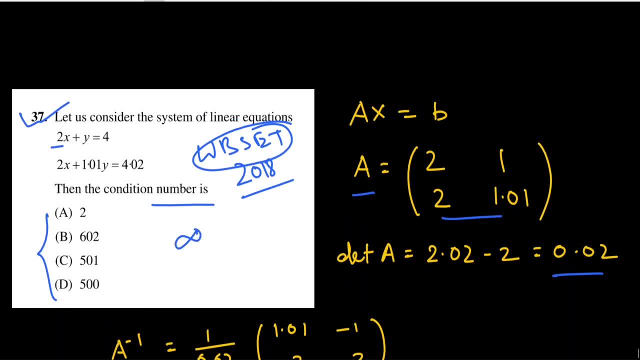 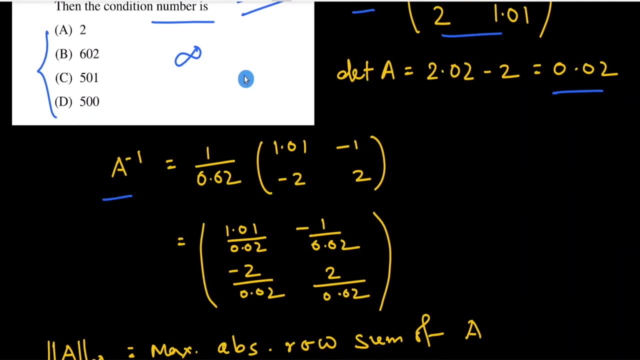 calculate the condition number using here infinity norm. now this is equal to calculate the condition number using here infinity norm. now this is equal to: gives 1.01 by 0.02 minus 1 by 0.02 minus 2 by 0.02 and 2 by 0.02, now norm of a. 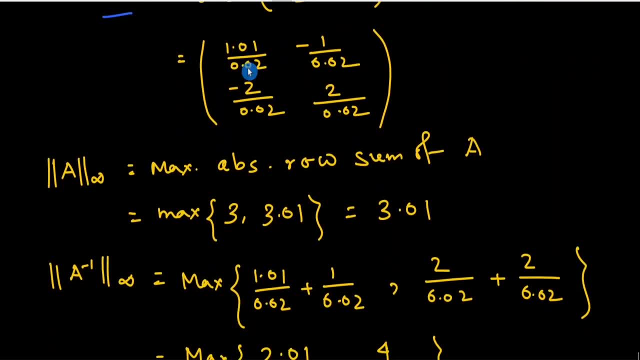 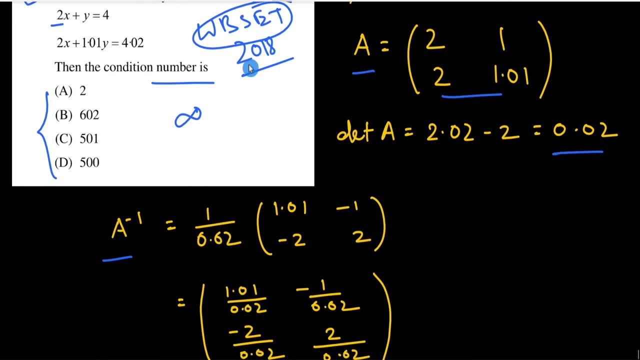 gives 1.01 by 0.02 minus 1 by 0.02 minus 2 by 0.02 and 2 by 0.02. now norm of a infinity: 2. Now norm of A infinity equal to maximum absolute row sum of A, which gives 3 maximum.